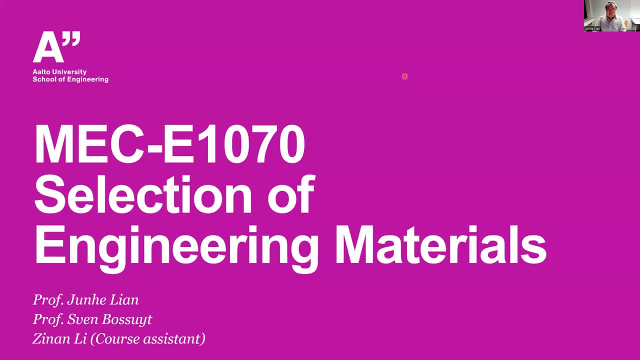 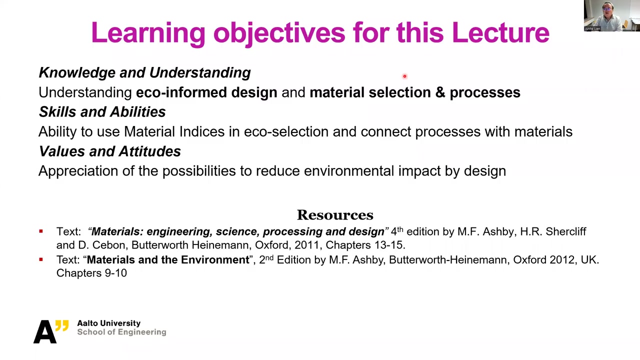 All right. so this recording is to provide additional supporting materials for students in section of engineering, materials for the UCO-related design and also the processes. So the learning objectives for basically this week is about first to understand the UCO-informed design and also to gather concepts of material selection processes. Yeah, we have been speaking. 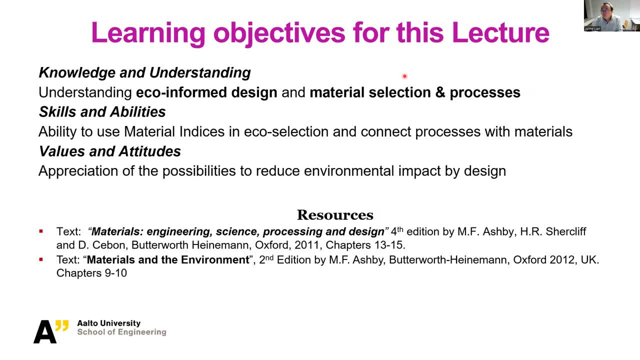 about material selection quite a lot, but you have to know the materials in terms of their mechanical properties are not just the single item we consider when we do the selection, as you have to consider processes, As we discussed before. for many cases we determine the bamboo as the best material. 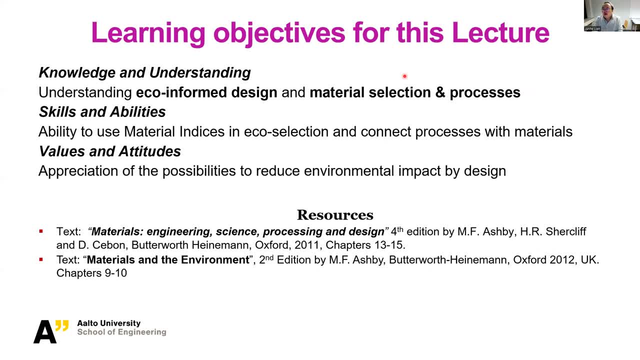 in terms of stiffness, even strength, But in the reality you suddenly use that in many engineering structures. By understanding processes, you will finally know what really the processes we can use to shape, join and finally have a good surface of our final product. So processes- 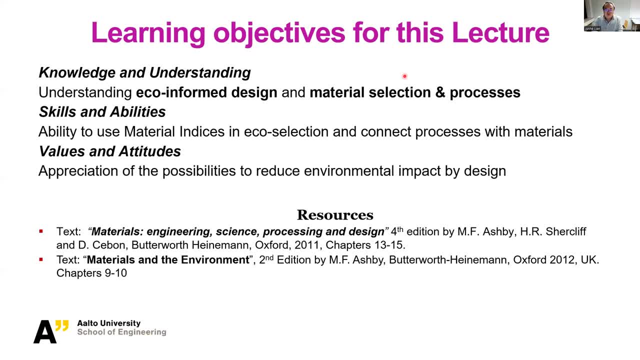 are also important. It's also an important chapter for us to always discuss and think of when you do the design And after the knowledge and understanding, we hope you will be able to use the material indices in the eco-selection. So this is a separate unit of the ADUPAC And to do the 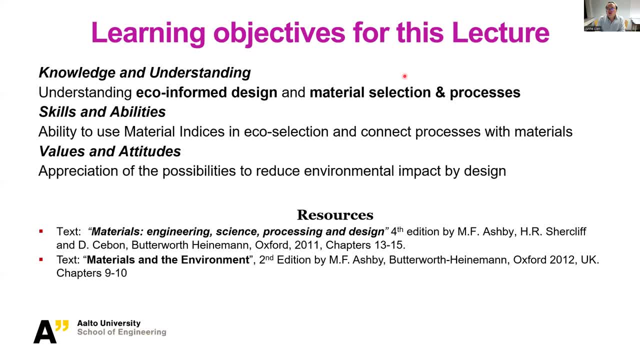 eco-informed design. that's the first skill And the second. you could also connect processes with the materials when you do generally. And finally, we would like you to be able to always use those skills and abilities and understandings in a bigger picture. You could always think about environmental related issues. 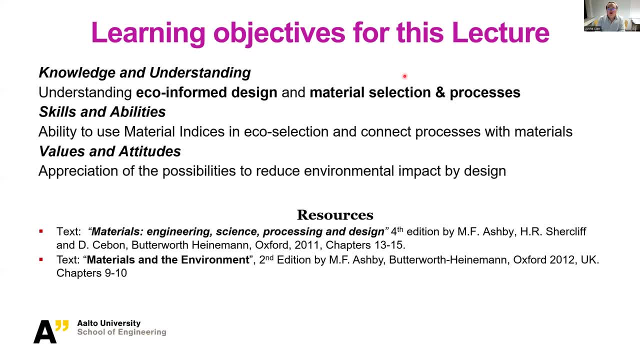 and impacts in terms of CO2 emission, in terms of energy use. It is becoming really a critical issue, Even nowadays. I think everybody knows what is going on with the geopolitical issues, So that makes all this kind of concern about environmental impact and sustainability more. 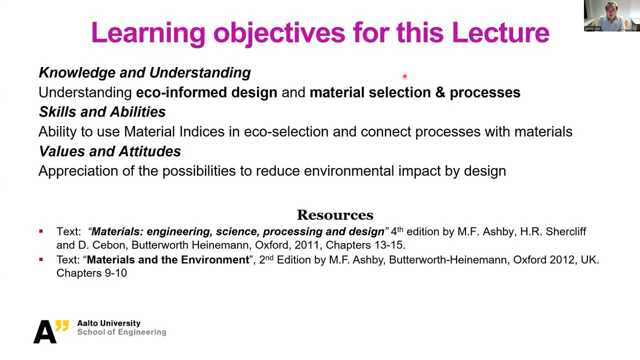 important when you do any kind of designs. All right, In the resources you have the textbook And in addition to that there are two books for you to also read if you are interested in this topic. The first is Materials Engineering, Science, Processing and Design by Ashby, And the second 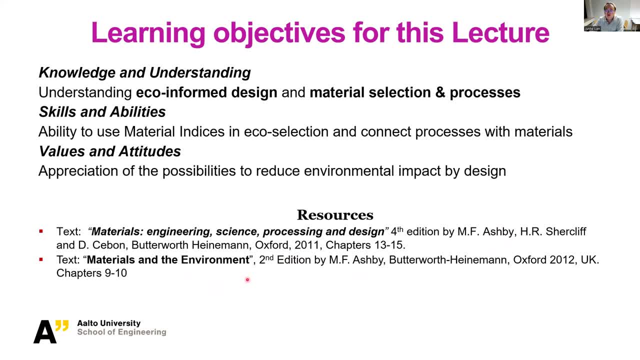 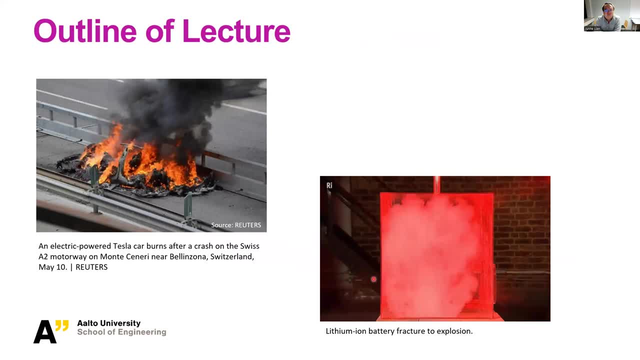 is all reading very much dedicated to materials and environment, also by Professor Ashby. All right, So what is the outline of today's lecture? So before we go to the lecture, the outline, I would like to already show you two pictures. 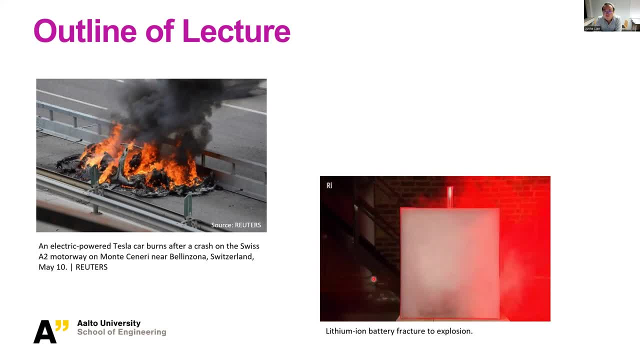 which is not directly related to kind of impact or environmental impacts, environment and or let's say, energy use, but it's a slightly remote related. so I think these two pictures are good for for us to get the introduction about the general, I mean, let's say, motivation of 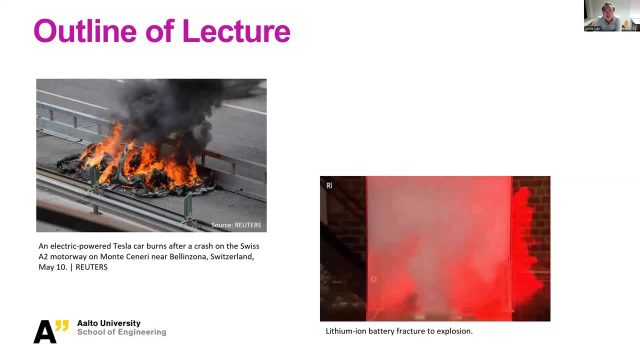 where we're doing right now in the energy sector, exactly. so you can see, on the first one on the left, I'm showing you one, let's say a burnout of Tesla, um Model S. yeah, the accident happened actually in 2018. um in May it happened in in Switzerland. you can see the accident was pretty. 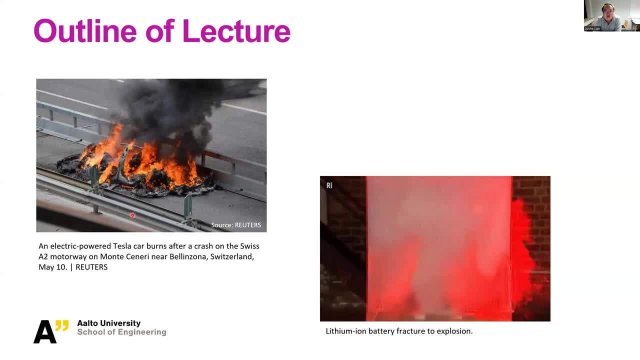 simple. they- the Tesla Model S- basically had a crash on the barrier, this kind of steel main thing, and that really caused some very severe damage to the batteries and that battery finally induced a, a thermal runaway and also and a big fire. so this is one very burning issues for electric vehicles. yeah. 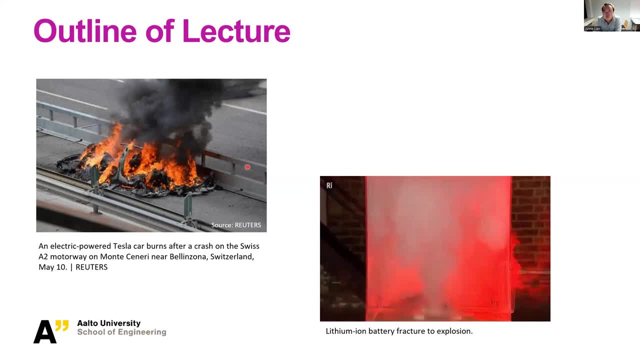 so the safety issue is very, very big, big, important issue for them to consider in the in the use. so, on the right, I'm showing you one battery. yeah, right here you can see this is a cell phone battery. yeah, it's much a smaller one and, and before before this, the battery was getting all this smoke and so 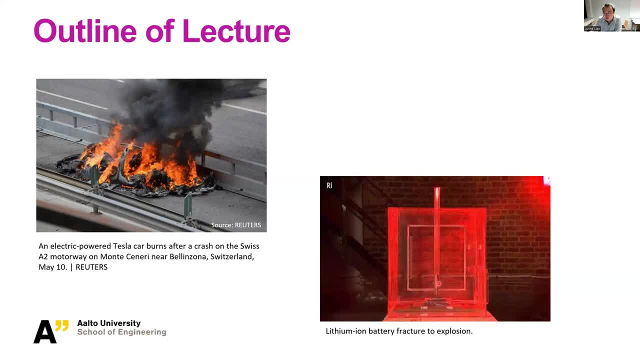 on. if you just pay attention a little bit, you see there's a kind of middle and it's bigger than a middle, but it's a very sharp tool with a little bit impact. you see that the height is really small and this little impact with this small machine you can see, cause really a significant damage to 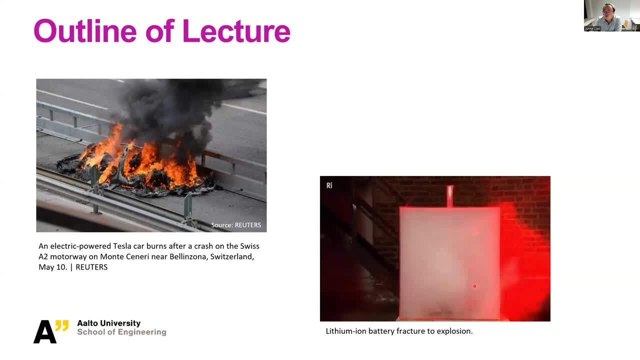 the battery and smoking here and also thermal runaway. I mean, if it's more severe, you can imagine that will trigger some explosion or big fire, like we have seen from this Tesla. so this is a little bit challenging for for the electric vehicle, of course, but what is the connection to to our course? yeah, I'm showing you really bad things. 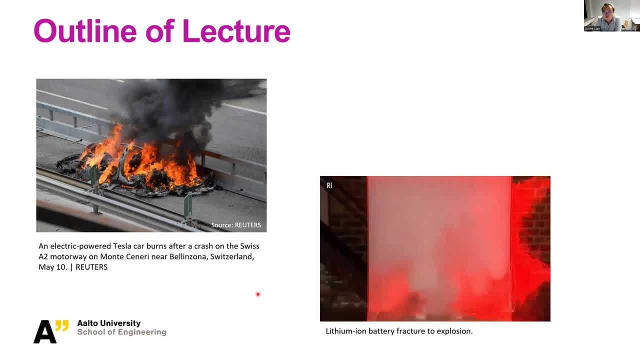 about these, about batteries, but why we are still using them, why we are still promoting them so badly and in um, basically all the sectors. yeah, and then I will show you a little bit about this. so this is the outline of today's lecture. so first we will show you. 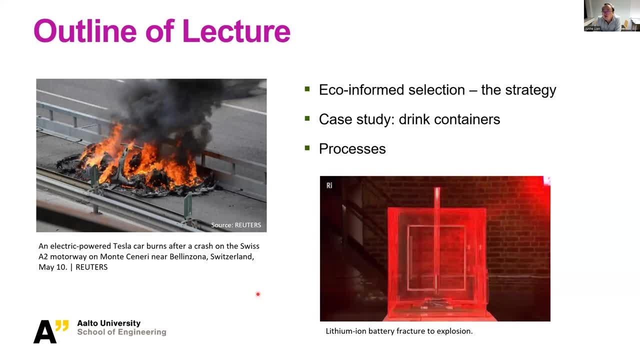 um the strategy, about eco-informed selection, and before the strategy, I will also tell you why we need to: um basically consider the energy use, can be considered the CO2 emission so importantly and to promote all the use. of this I mean UVs, even though they could have really significant. 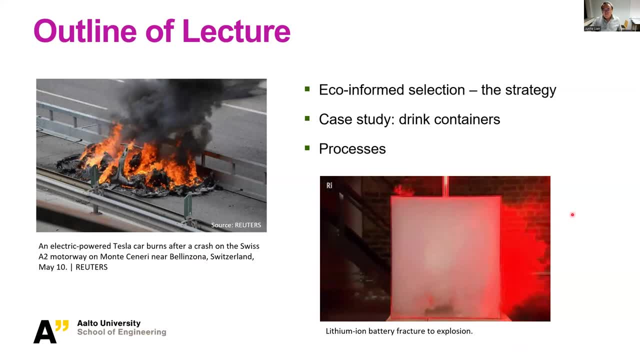 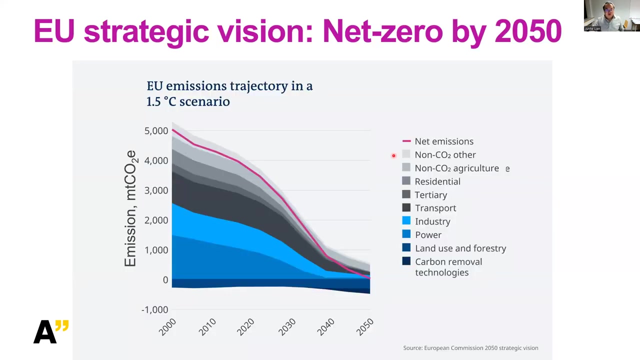 um, kind of dangerous events, and after that we'll go to a study and it's about drinking containers. yeah, it's a very interesting one. and finally, I will talk a little bit about processes. um, but that will be rather short. I think you can get this sense pretty easily from the book. all right, let's move to the first concept. so, and this: 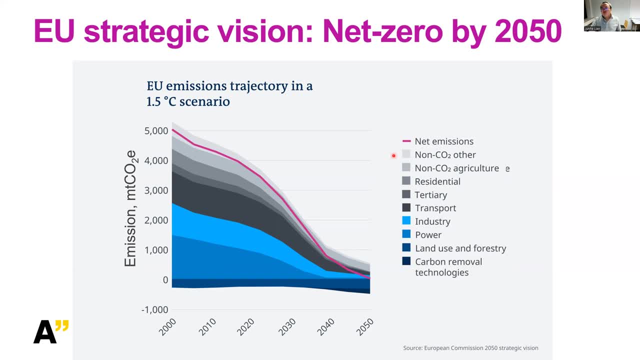 is about this EU strategy vision about net zero of CO2 emission by 2050.. yeah, I think most of you have heard this. 1.5 degree C scenarios, yeah and uh. if you don't know, I could explain just shortly. you know this is a scenario we kind of. I guess more than 200. 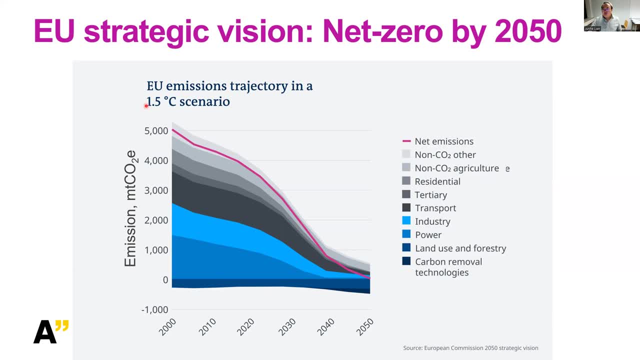 Nations agreed during this um, Paris agreement: yeah, in 2015.. and the the the data agreement is. it says we cannot exceed a 1.5 degree C global warming by 2050.. otherwise we will really enter very serious problems. yeah, so the, so this simply is called Paris agreement and uh, or also called 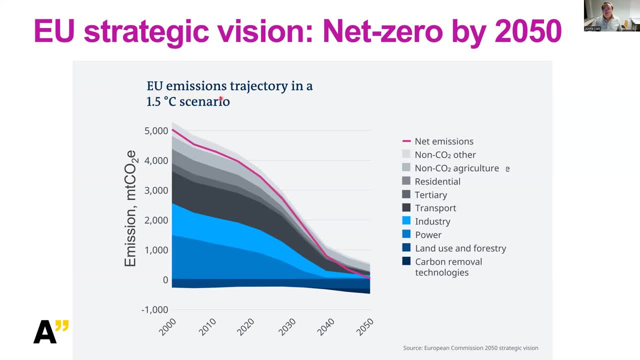 1.5 C and 1.5 degree C scenarios. yeah, so this is the name of it and what it means in general and basically, this requires us to reduce the CO2 emission. you know the global warming is mainly caused by greenhouse greenhouse gases and CO2 is the major issue of there. 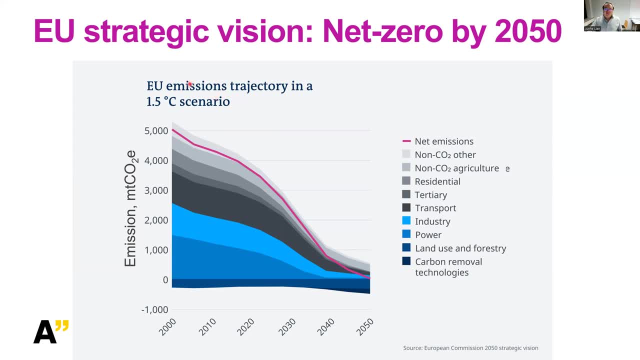 and so just to meet this kind of strategy vision, yeah, or this kind of requirements, and you made the following, basically strategy here. so if you look at the current emission of CO2 and now we have in the Europe, now we have a annual CO2 emission if you just take a look at 2020. 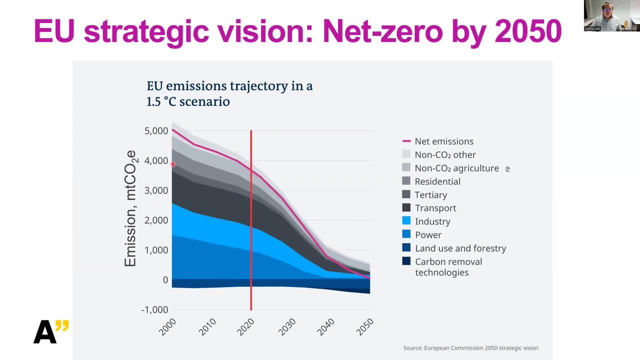 because this is actual data. we are close to, basically, 4 000 million tons per year. yeah, so 4 000 million tons is quite a lot and if we want to get to this Paris agreement- um, realistic, yeah, we have to reduce this significantly. that's, the increase of the global warming everybody has seen is dramatic in the 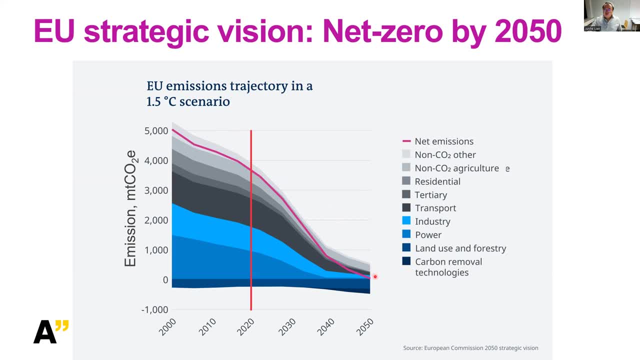 past years and we want to reduce you, reduce it to a final situation which is so-called not zero. so not zero means the plus and minus of CO2 will be zero. so you, you know um plants can take CO2, make them negative, but we also want to encourage other Technologies basically to to observe CO2 and and gave something. 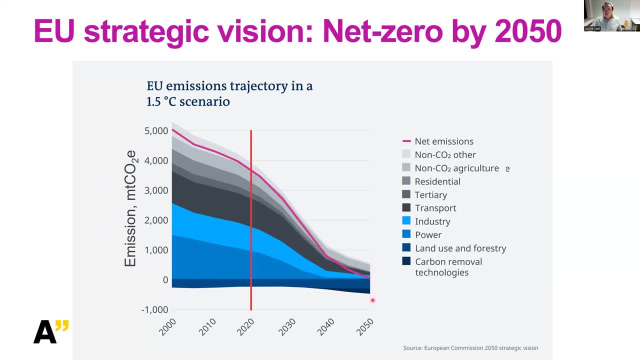 else you know. so that's why not zero means doesn't mean we do not emit CO2 at all, means we emit CO2 in an equal amount as the amount we could handle, just to observe. so this will be not zero by 2050.. and you see, this is now and this is 2050.. so 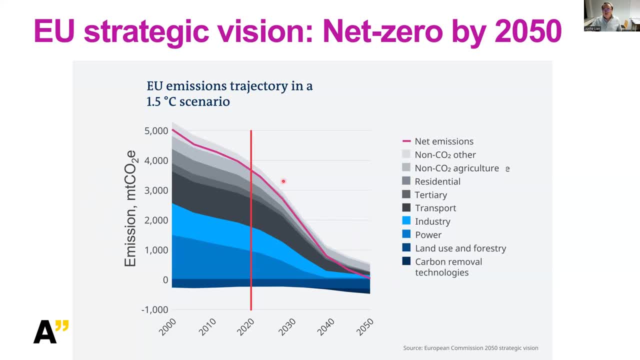 they. um, the task is is very, very hard. yeah, if you just pay a little bit more attention, the very big contributors to the CO2 emission actually are these three guys. yeah, you see, this is transport and the light blue is industry, so general industry and like PowerPoint and 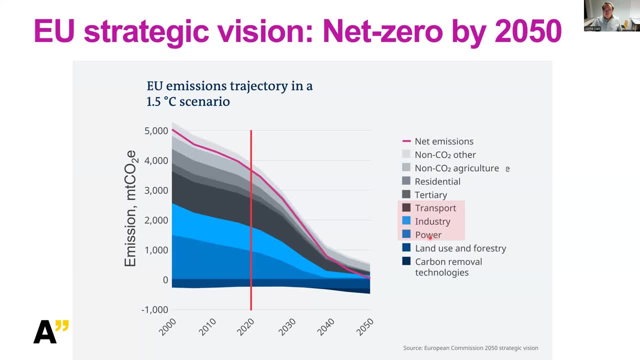 still making all this industry and- um, I'm sorry, the dark blue will be really power plant and power related CO2 emission. You know that's a big issue for us: to get energy and also to burn to emit CO2. So these three are critically related to the CO2 emission. 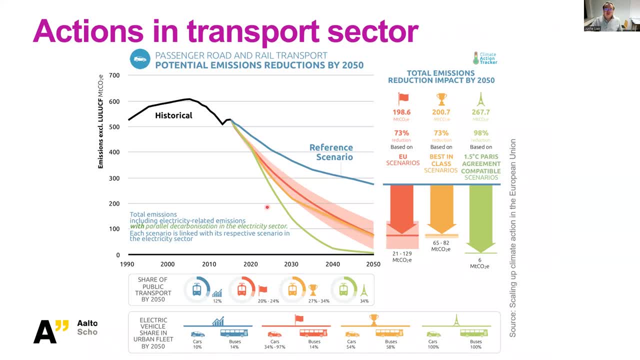 If we just look at a little bit more detailed sector, which is the transport sector, and here I'm trying to explain why we need to go with the EVs, so finally, to let you know why we have to do that. So this is a diagram rather complicated. 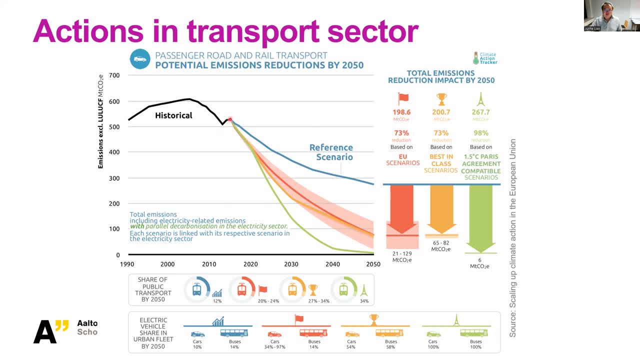 but if you just look at it, so here's now, or a little bit earlier than now, and this is our CO2 emission, basically for transport only. You see, this is around about 500 million ton CO2 per year, And that's, that's quite already a big fraction. 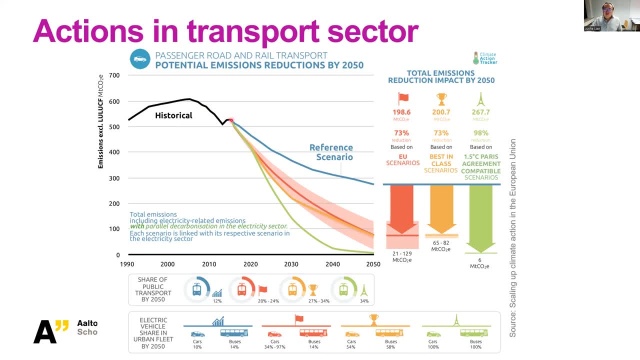 as we see from last time, And now if we want to reduce it. so you see we have different scenarios. I don't need to look at all of them. It's really in very detailed analysis. The reference means basically, if we don't do anything. 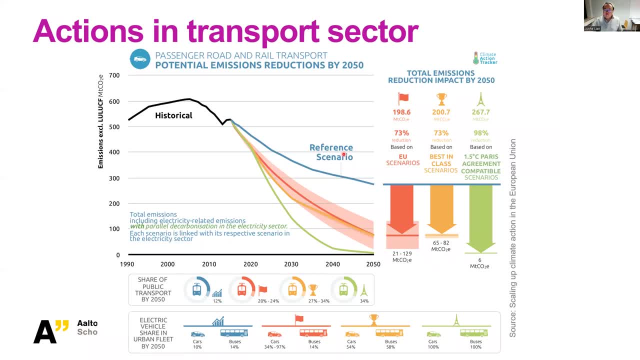 I would just let it run. It don't impose any, enforce any kind of policies or technologies. we specifically relate to and say CO2 control or energy and sustainable energy use, And this is what we'll get. We will generally get a little bit less CO2 emission. 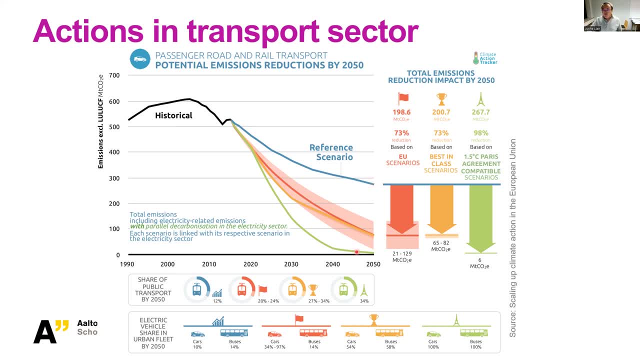 but this is far beyond the zero emissions right And if you work a little bit harder in between, like the other scenarios like this, you can get a better. but if you want to meet the Paris agreement, so the 1.5, 1.5 degrees C. 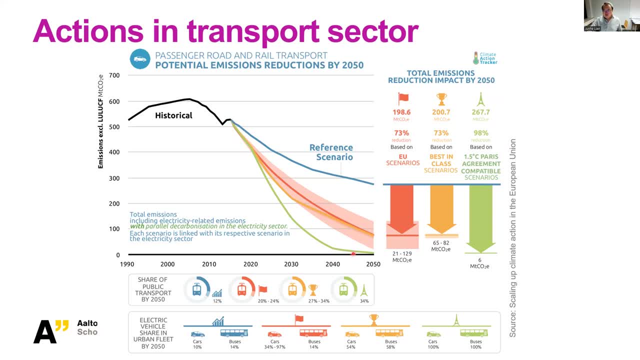 we actually need to follow this green. So, this green, this is our goal to to basically reduce all this 600 million tons CO2.. And what is the reaction? So the reaction, basically, is this too, We need to increase a lot share. 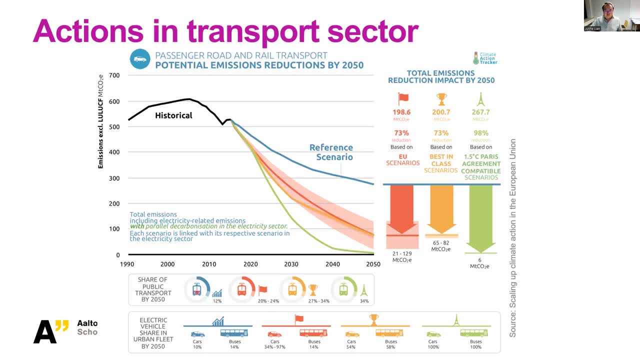 of the public transportation use, As at the moment we have run about 12% and we need to and we need to get 34%. I think this is really getting pretty good, especially in Nordic countries, and public transportation is getting very much in big share. 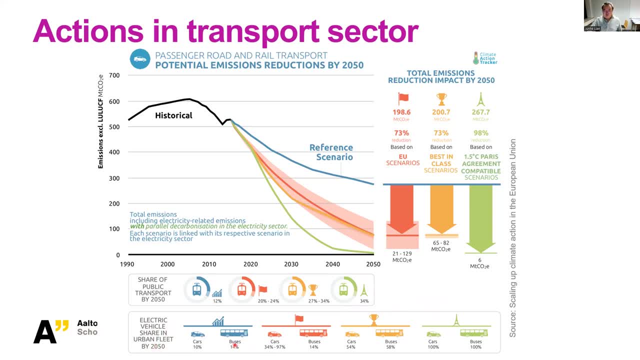 And the second measure is more critical because we have to also consider, you know, the urban fleet, so basically cars and buses, And if you want to meet the Paris agreement, meaning we will have to build the electric vehicles- doesn't mean always electric battery. 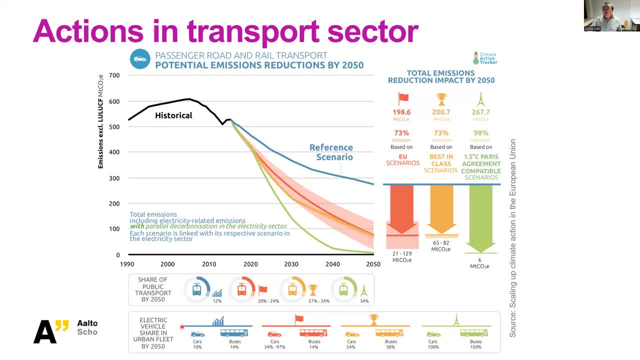 or lithium battery driven. It could be also other kind of few cells and so on, But the bottom line is that the vehicles cannot use fossil fuels that will generate the CO2. And this has to go a hundred percent, And so you can imagine in about 30 years. 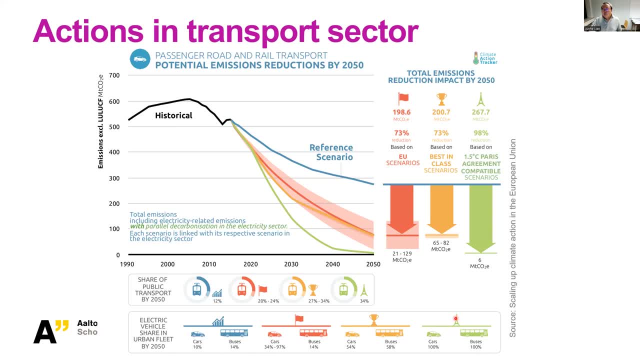 in the kind of urban fleet you will not see any. I mean cars running by, you know, diesel or gasoline. So this is something we have to imagine right now, otherwise we'll have big trouble with the climate, And this is also the fundamental reason. 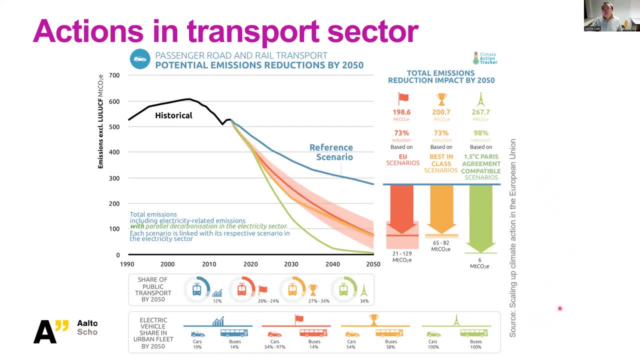 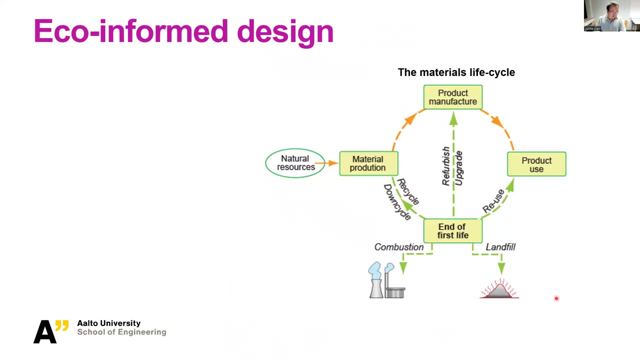 why we have to go with electric batteries in the vehicles Or, in general, just electric driven vehicles. All right, Now it comes to the design phase. So I think that was a good motivation for you. Maybe some additional information for you to realize. 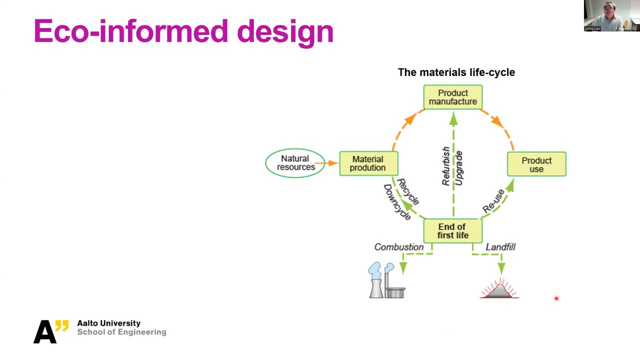 why we're really promoting the kind of green energy and also green use of energy in different industries. And here I'm showing you a diagram. just you know a diagram. So here's a diagram of the different industrial areas. I want to show you the one that you see here. 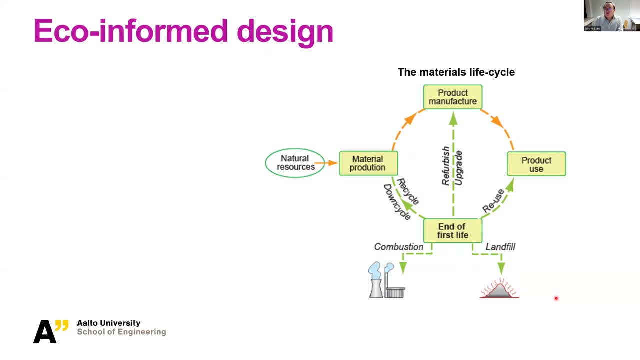 And these are the sort of different industrial areas. And this is a diagram And it's really just to consider when you really go through the material selection field, when you go to the, let's say, the product design, what is a life cycle of material we should consider? 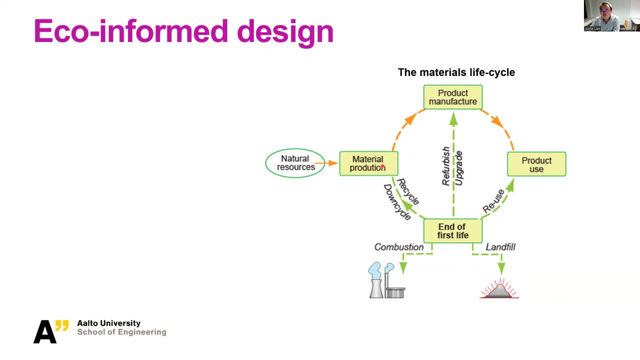 Yeah, And the basic information is we have material production and we also have the product, let's say manufacturing. So the cycle goes from here. So we take the natural resources, yeah, everything we have. So you can see that there's a lot of different materials. 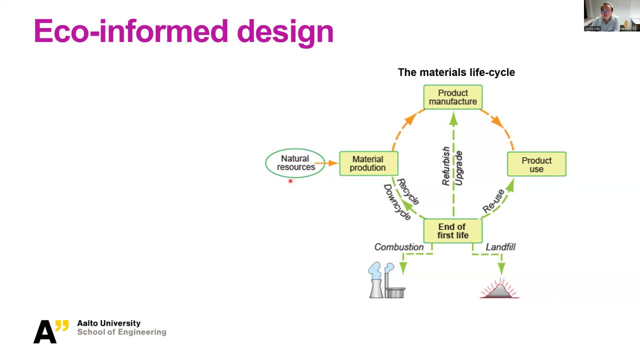 If we think about aluminum alloys or steels. you know you will take the ores from the earth. basically, yeah, Then you go through already a long process. you know iron making, steel making and coat rolling, detrimment and all these processes. 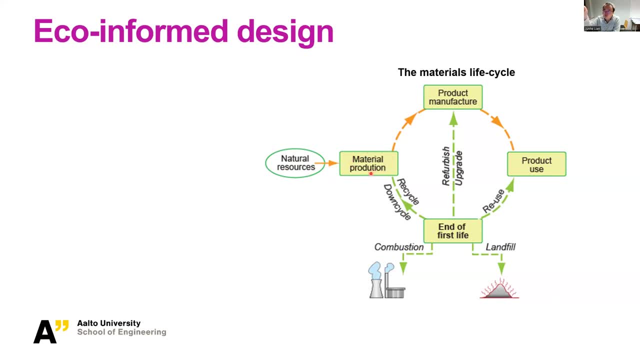 You basically get your raw materials, yeah, in terms of sheet, in terms of wire, And if you want to produce, let's say, a car, the body of the car, then you need to go through the product manufacturing procedure, basically by stamping by all the different kinds of shaping. 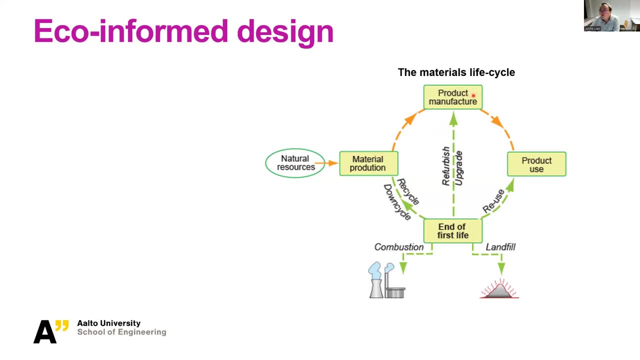 And then you finally get the body of your car. And then you get your car and you're going to use the product. Let's say you're going to use the product for 10 years, 20 years, And then the product is not in a very good shape. 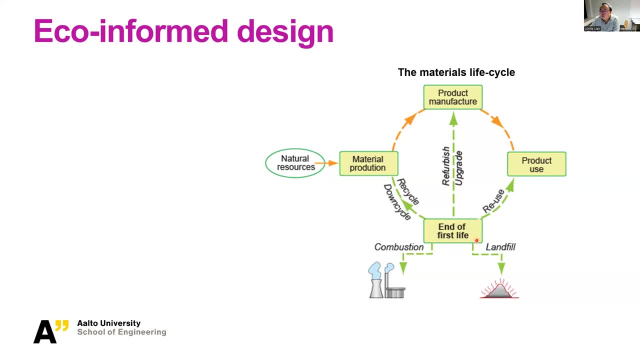 That is determined as the end of the life. but you have to pay attention, it's the end of the first life, yeah, So after the end of the first life, some of the products- yeah, will basically go into these two fields. 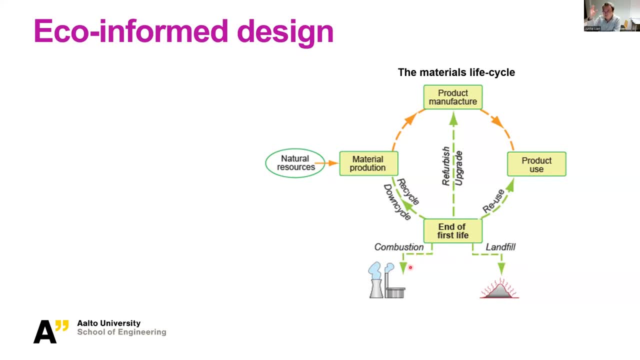 So the first is combustion. you see, most likely for our plastic kind of- yeah Garbage and so on, yeah, They might have to go to such a base And if you think about nuclear-related kind of waste and so on, they will have to go into landfills because we basically have to end their life right now. 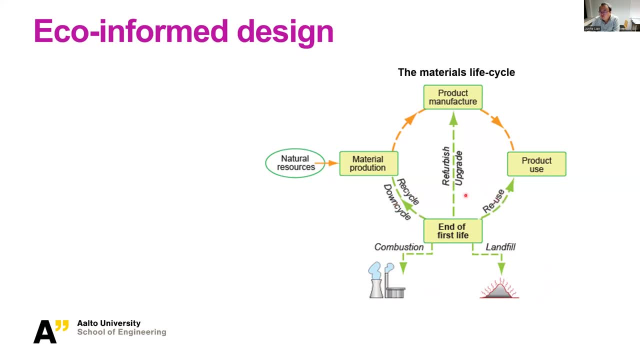 But for others- and we would like to promote the most of the others go to these three kind of directions. So after the end of the first line we want to give The second line, basically So they can be recycled or downcycled. yeah, unless you deal with lots of, let's say, the can of Coca-Cola and all the others. 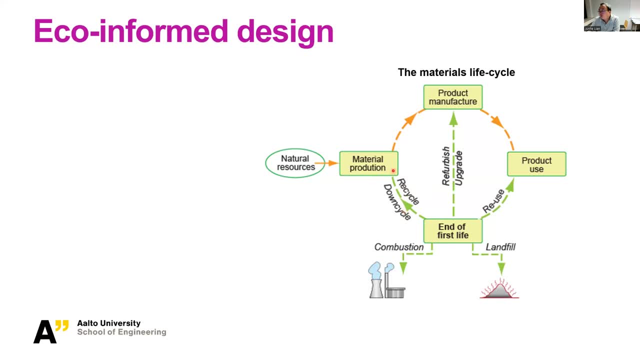 So they will be recycled, basically, yeah to the material production. yeah, So you will use them to reproduce some steel, aluminum alloys, things like this, and you could also get a basically an upgrade on refurbishment. 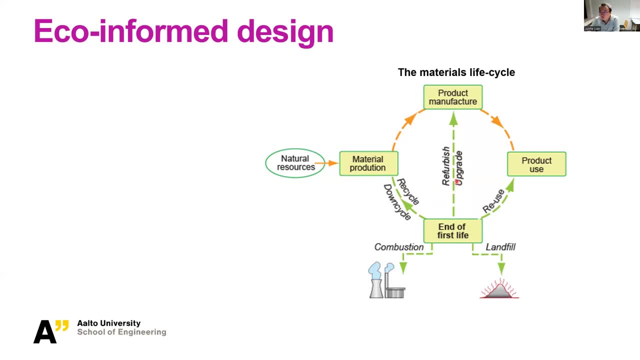 For example, for a second-hand car- yeah, you could do that, or you can basically to reuse it. yeah, so directly use it for the first, after the end of the first line. So these are the three directions we would like to think which are doing positive things. yeah. 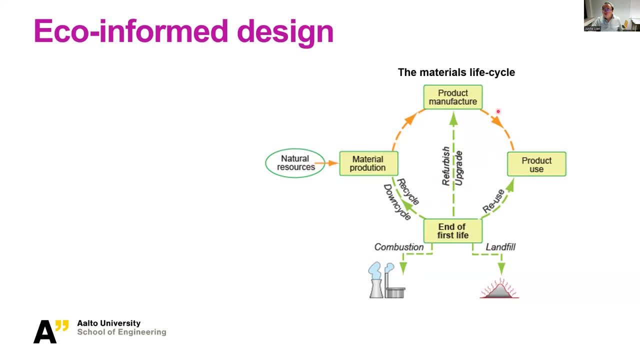 If you just look at all these orange-colored arrows, They're consuming energy. you know they're consuming energy. they're emitting CO2, most likely, and after the end of the first line, okay, we're not even here- we're probably still consuming energy and also emitting CO2, yeah, and they should have the orange as well, actually. 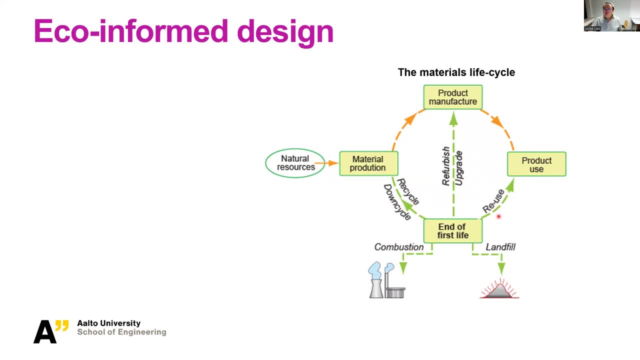 But these three- yeah, these three green arrows- and they're doing positive, So they're not consuming energy because they are contributing positively to our material use and to our CO2 emission. So these are the things we should promote and we should think to when we do the design. 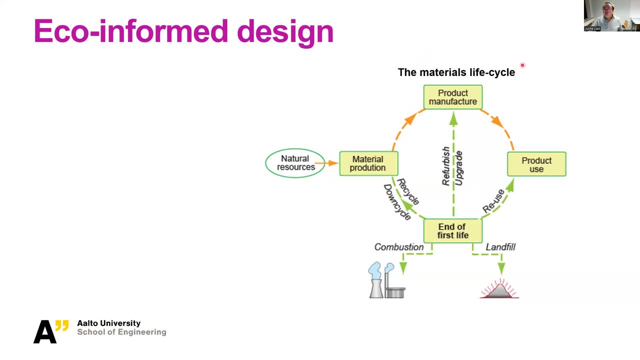 So basically this is the so-called material life cycle and you could have it in mind And why it's important? because you know they kind of equal impact that our product and all the material will make will be decided already- 80% during the design stage. So when you design your product, when you do the material selection, 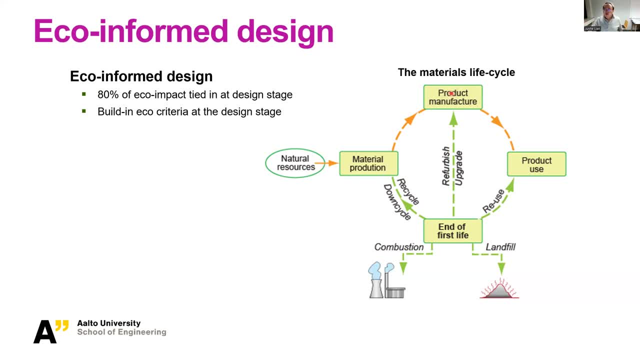 at this phase, at the design phase, you choose the material, you choose the processes and you choose the use and you probably already maybe not choose, but by all your choices, the end of the first life. the choices are also made Now. that's why it's critical when you do, 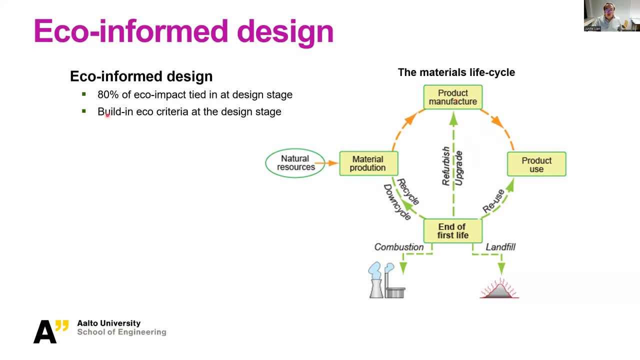 the design. you need to consider this whole picture And 80% of the equal impact is already determined during the design phase. So that's why we need to have a tool Basically to estimate what is the equal impact in terms of energy use, in terms of CO2 emission. 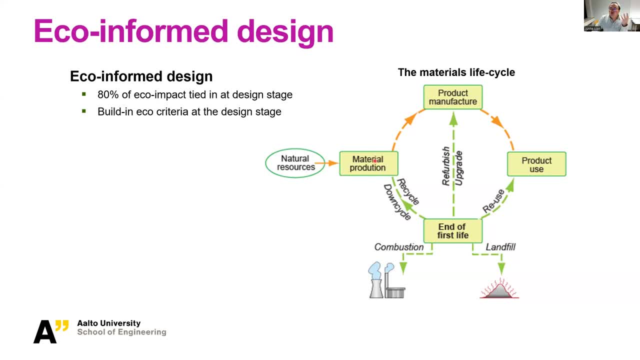 and this will give you certain information about the equal impact and that will also basically design how you do your material selection afterwards. So this is basically the strategy we're going to do and why we need to have the equal informed design process. So that's why we need to have the equal informed design process. Basically to estimate what is the equal impact in terms of energy use, in terms of CO2 emission. and that's why we need to have the equal informed design process. So that's why we need to have the equal informed design process. So that's why we need to have the equal informed design process. 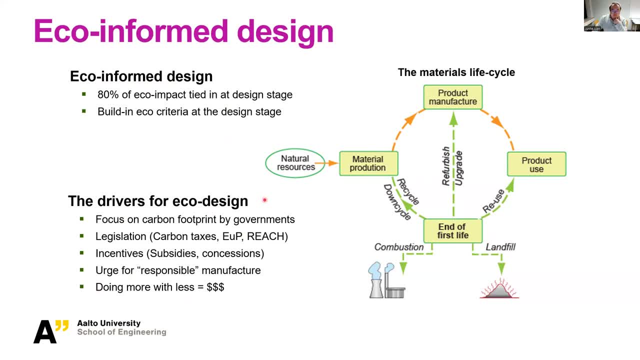 Now let's discuss some of information about product quality like: Oh, we have suitable filters in our field of high energy and the product quality as well. the efficiency for each material was in the group pairing my presentation at the end. So how can we develop it? program. 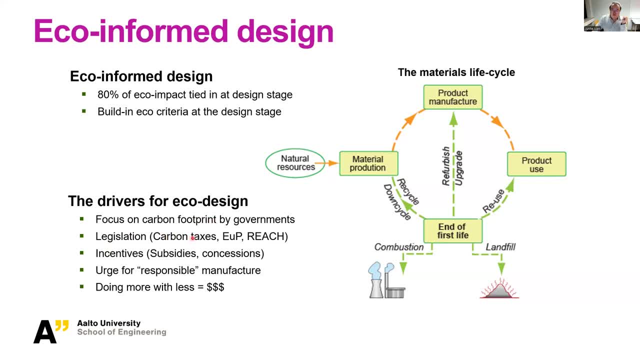 therecipit and material selection And, as you can see, the other instruments like government promoted CO2 footprint tracker and also legislation about CO2 carbon taxes and so on. so basically they're all forcing everybody to consider the equal impact. 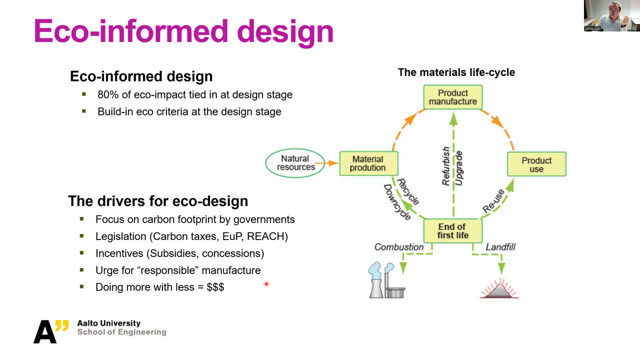 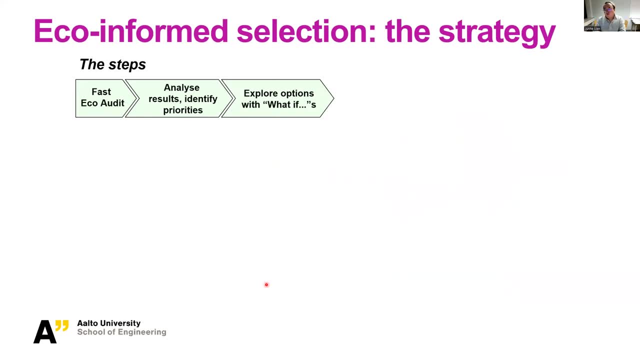 And this has to be considered during the design of your product. And in the next I'm going to show you how this strategy- when you consider the silvery emission in the design phase- And basically it follows the following steps. You could get this from the book in more detail. Here I'm giving you a very rough 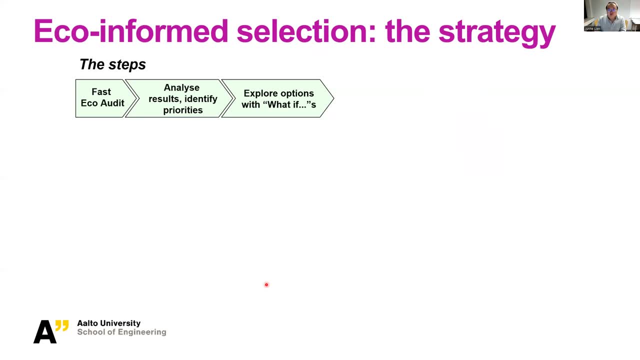 let's say introduction about it, And there are a few steps first already. So we need a tool, as I said, And the tool is called Fast Eco Audit. Now this is included in the Greta Edipack And you're going to use this to analyze the results and identify certain priorities. 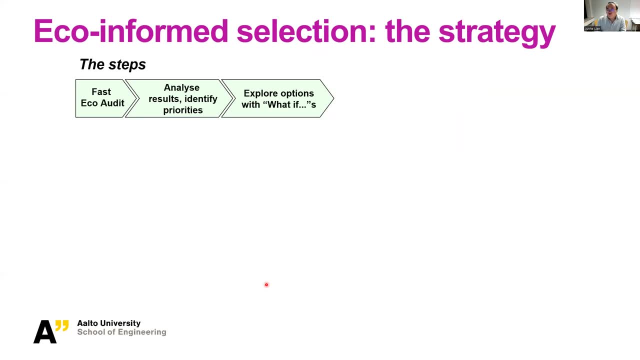 And then you explore, basically, different options of your material selection And say: if we use another one or this one, can we get a better CO2, sorry, equal impact. And to visualize, here is what you see. So this is the so-called energy that you're going to use in a material. 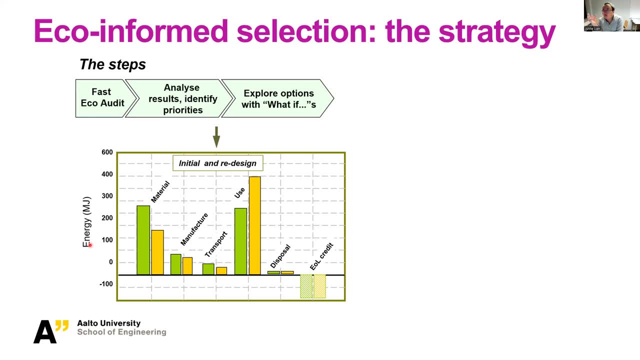 line. So it's kind of an integrated measure of the impact to the equal impact. So the CO2 is part of it as well And, as you can see, we will see all the phases as we discussed before And in the last slide. this is the energy that is going to go into the material And then the CO2 will be. 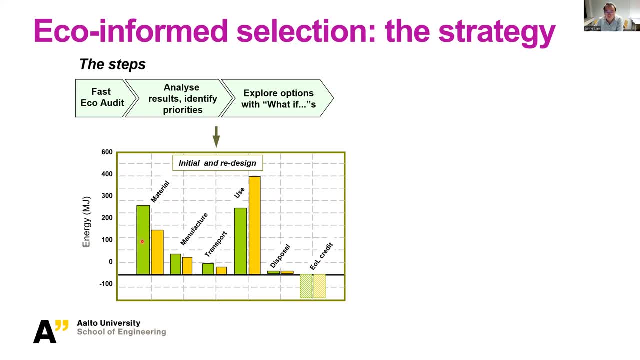 multiplied into this material life cycle basically. So you cannot just think about the material production. Now, this is the material production. So, for example, if here is steel, here is aluminum- yeah, And maybe you know, in the production of steel it is a little bit larger. 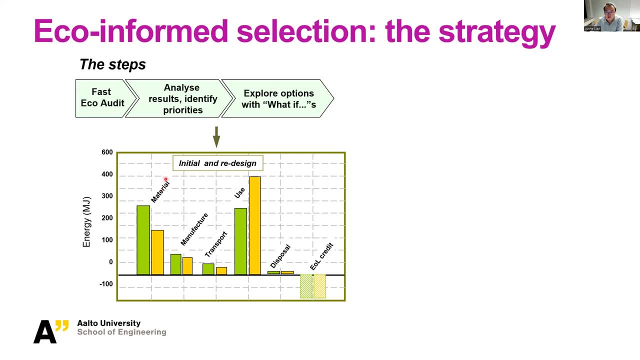 scale, maybe more expensive and contains more energy. not more expensive when you do the material production. But you cannot only think about the material production. Yeah, You have to think all the following phases: the features like manufacturing processes and transport, and the product use and disposal. 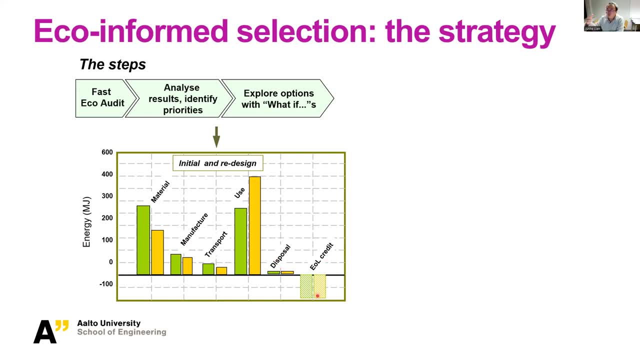 And this is end-of-life credit. As I said, the end-of-life credit will be inactive, so it will make your energy consumption in general lower. So that's why, if we can identify materials which could contribute a lot of end-of-life credit by reuse, by recycle, this is always. 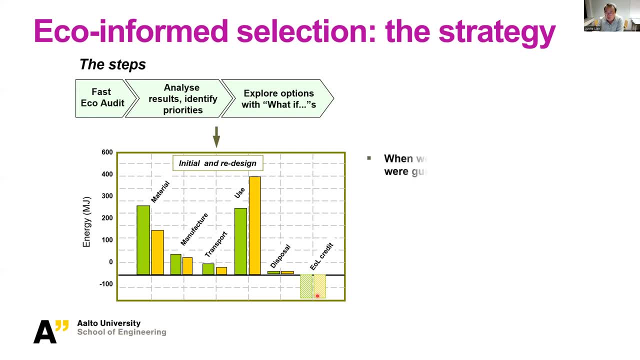 very much encouraged, And after that you can just explore. As we discussed here, these two materials can go basically more If we use another one. is it better, Can it be more systematic? And then you can just apply the selection methodology to. 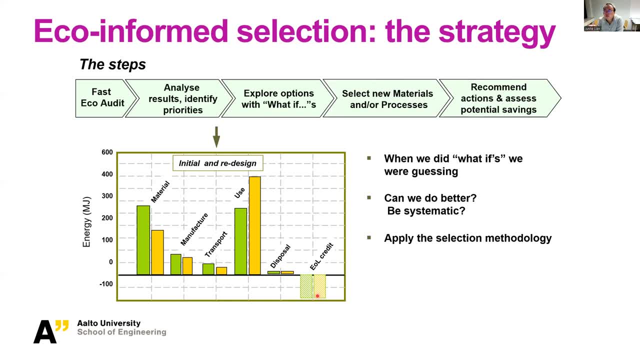 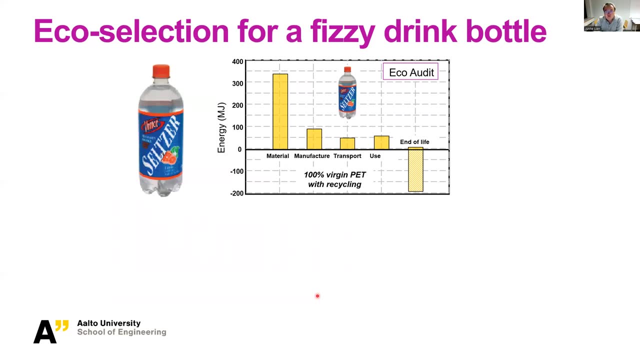 finally select the new material and processes and then do the recommendation of the action and assess the potential savings between a bunch of materials you would like to think about. All right, so that was the general strategy. I think that was easy to follow. You can also get more details from the book. Now I'd like to give you one example. 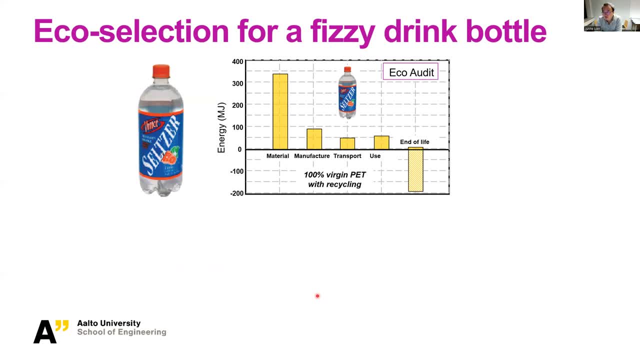 which is a quite interesting one. rather easy, but it's really easy. This really integrates many concepts we have learned in the few weeks ago. and also to think about this ecoaudit or eco-impact design. So the example is about the eco-selection for the fizzy drinking bottle. so looking like this: 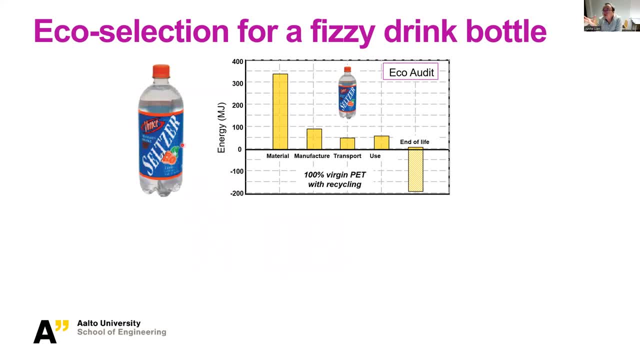 It's not just the normal bottles. this will be the bubble water, yeah so the water with gas, and that gave us a certain requirements of, let's say, strength requirements of the materials you will see in the following. and now we want to think about how can 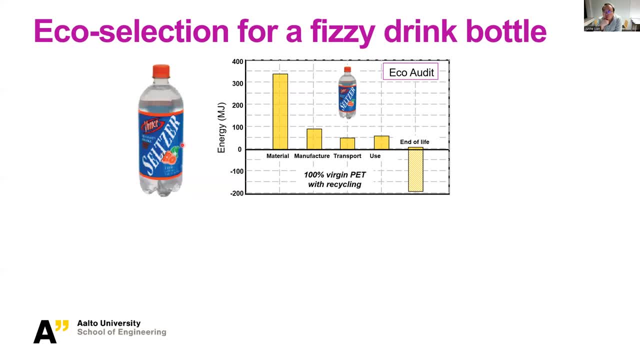 we do a eco selection, so the eco-friendly selection. so that means we need to minimize the embodied energy. that's the thing we want to consider and you know how to do it right. the design brave is like. we prove three credentials of the bottle. we want to improve the. 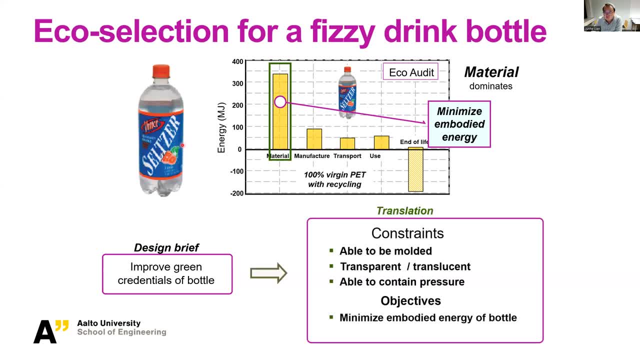 embodied energy and then we can basically translate it to constraints and objectives. so the constraints for such a bottle design is basically: should be able to be molded and transparent or translate. you know. you want to see what is inside, what is the color if it's just water or cola, and one of that it should be able to contain. 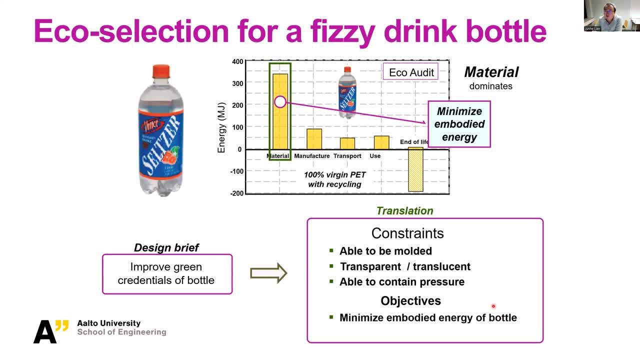 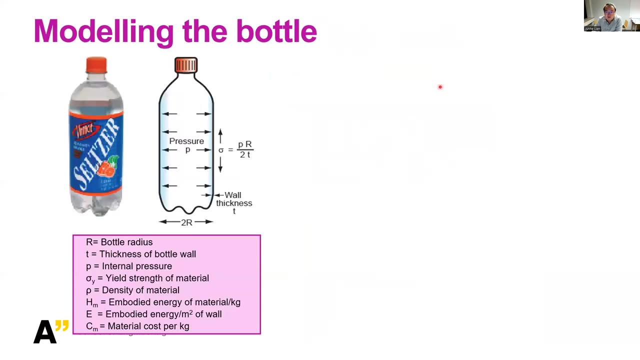 pressure? yeah, because we want to have the, the water with gas, and objective is simple. so we want to be more eco-friendly, we want to minimize the embodied energy of the bottle, basically using the um tool. so here is a little bit about this calculation, because we have one constraint. 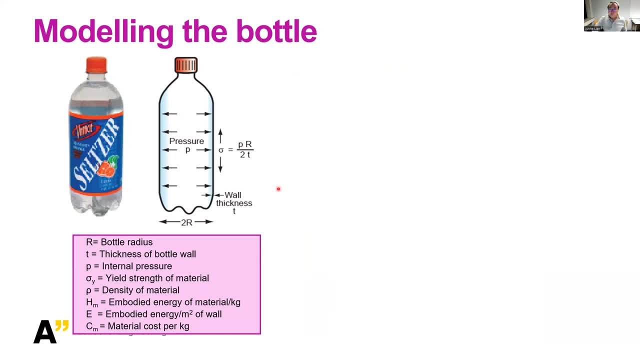 which is about to contain certain pressure. yeah, and you should know the pressure and how this pressure will be related to our material requirements, right? so here i'm giving you all the operations of the symbols and you can see the pressure. yeah, by very simple mechanics. the pressure can be basically expressed like p: the pressure here. 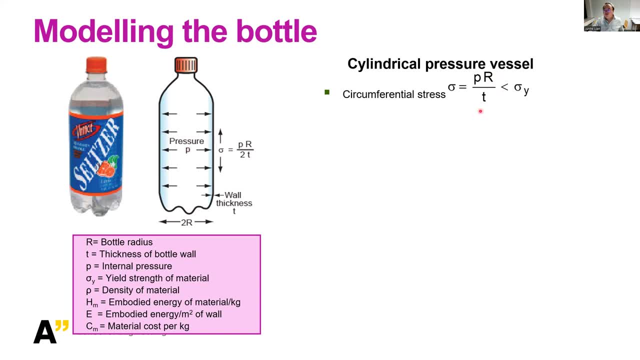 and times r. so r is the radius of the bottle divided by t, the thickness, and this will be the strength. yeah, the, the circumstantial stress of the bottle. and, of course, if we rely to the material to contain certain pressure, means this strength of the material has to be small. 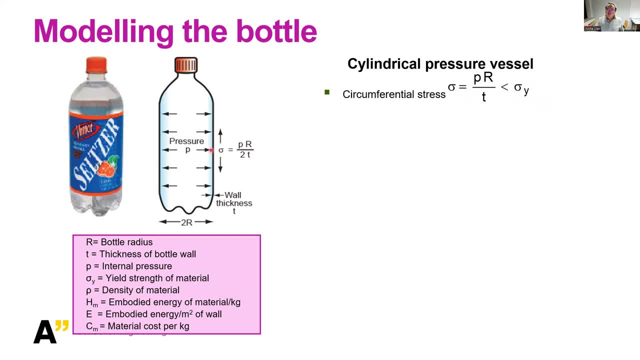 than the yield strengths, right? otherwise the material will be having positive deformation. that will be already considered as failure of the ball. yeah, all right. and then we want to calculate the embodied energy of the bottle, right? so we don't want to get the whole bottle, we just want to. 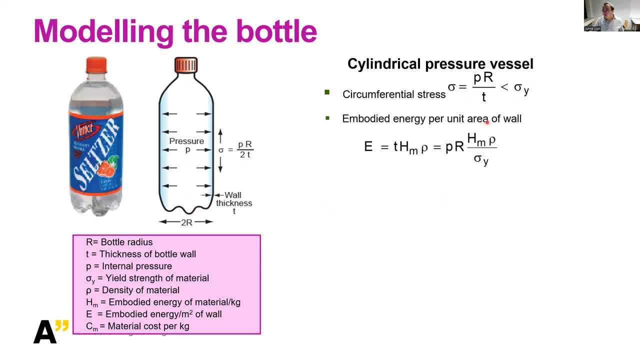 get the embodied energy per unit area of the wall right, because we don't want to change the geometry of the material. we just need to know how can we minimize the involved energy per unit area that you are already automatically minimizing the embedded energy of the ball. so this is a simple equation. 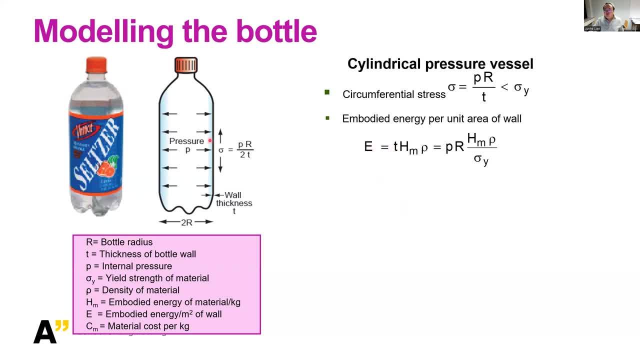 so you just you know the energy is equal to the thickness times the hm. is this involved? energy of material per kilo? yeah, and times the density role, and then you get basically the input energy per unit area. right, i think everybody could follow. and the next is basically you take 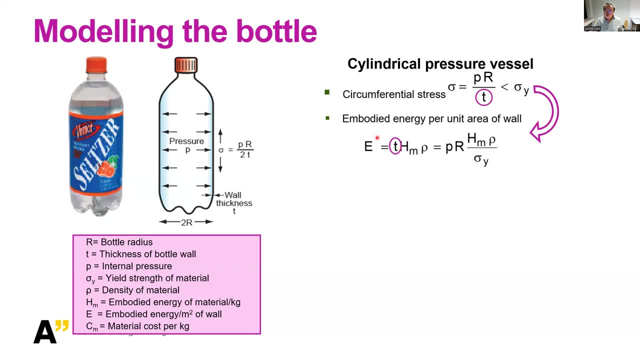 the t right. we don't want to have any geometry in this kind of material index formulation and we take the t from this first equation and replace the t by sigma y, p and r and, as you can see, here is our embodied energy. so if you want to minimize embodied energy, 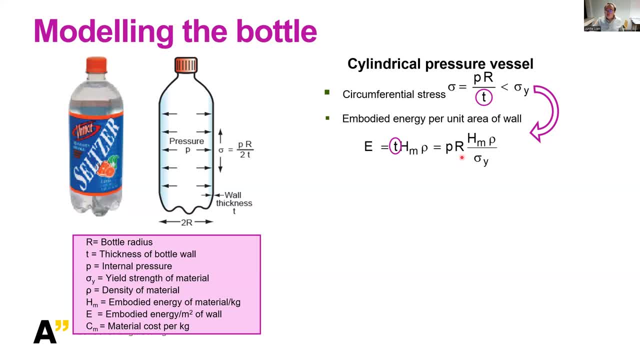 as you know, p and r, they are determined value, so that means we are basically minimizing this term, here, the whole term. yeah, now you can recall how do we formulate the material index. and we just take a reverse, because we don't like minimization, we want to maximize, so we want to. 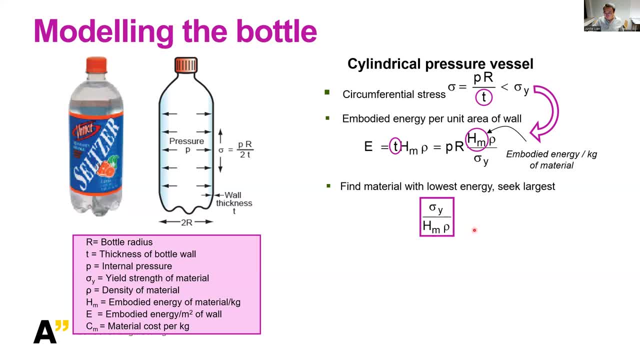 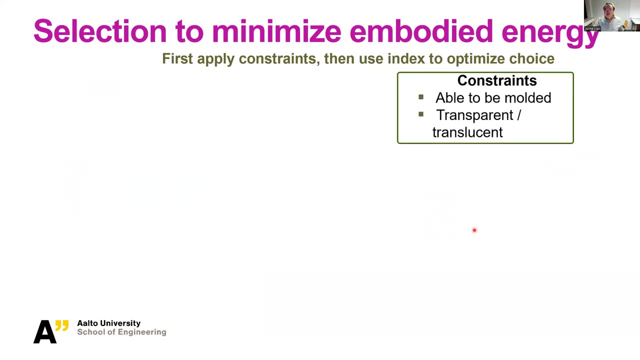 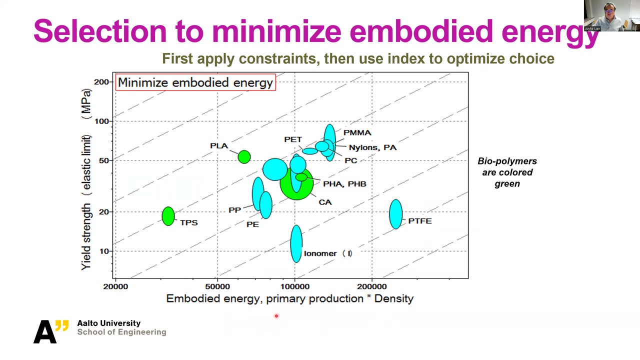 minimize sigma y over hm times, rho, right, so then you can just simply use our tool, as learned in this first task, to formulate a material index. yeah, if we just go fast here, you can see we can express our material index in this kind of r-speed diagram. yeah, you take the x-axis as embodied. 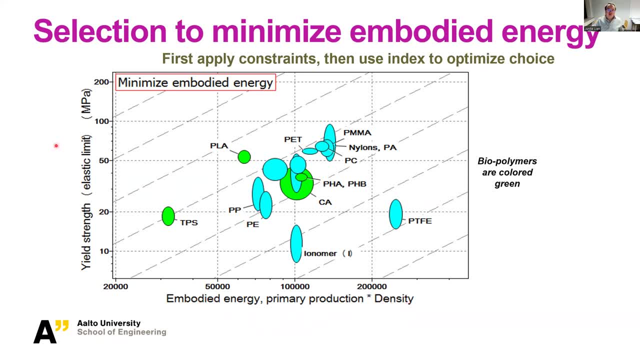 energy times, density, and the y-axis is the yield strength, yeah, and then we're basically looking for a, a maximum um asept here. so you can see, here the best material for this minimize the body energy is pla. now, so pla is a certain bi-polymer material, yeah, and so this screen wants dps also. 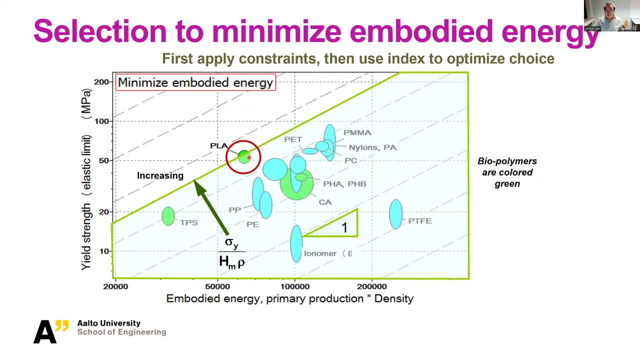 and you can imagine, that's why they're here, because they're really, let's say, um, environmental friendly, um, and it can't really get the minimize, the embodied energy. but if you know this material and if you know this business also in detail, actually for our bottles, 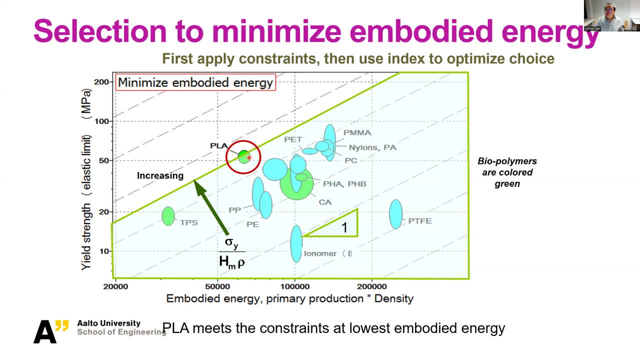 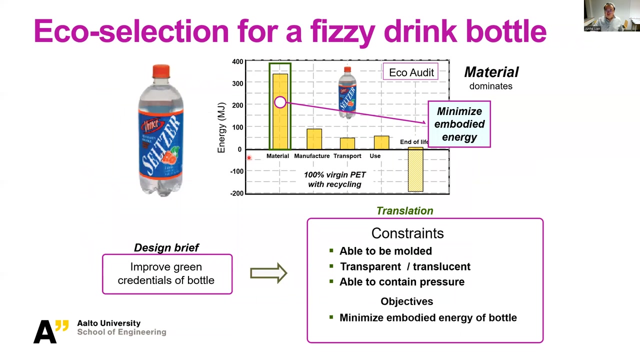 used. nowadays we don't use this pla so often. if you just take a look at your coca-cola bottle or any water bottle, maybe you can think that you can. you can take a guess: they are mainly made of pt. yeah, i mean you. you might ask: why is that, if we just recall the design principle? so 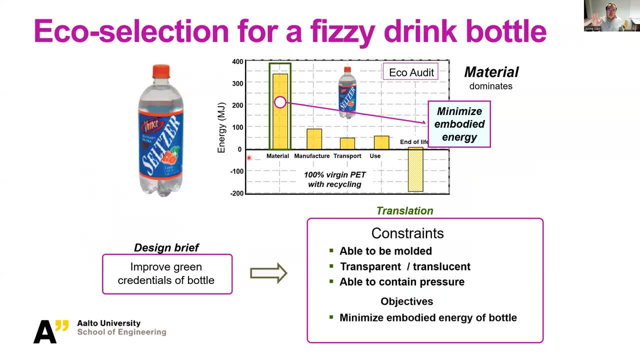 here i said, okay, we just want to do a best, equal, friendly selection. that's why we just want to minimize the embodied energy. but the truth is in the reality you can't minimize the embodied energy. you cannot only go for that right, you can, you can imagine. we have to also think about the cost. 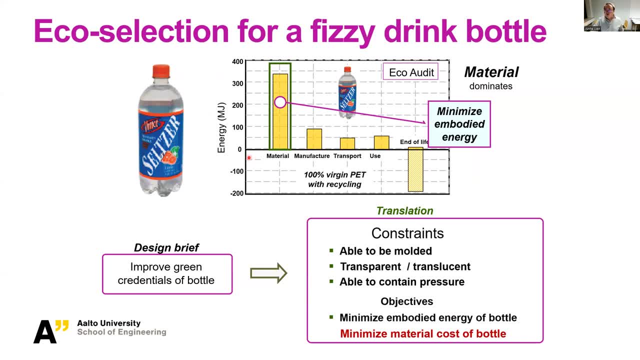 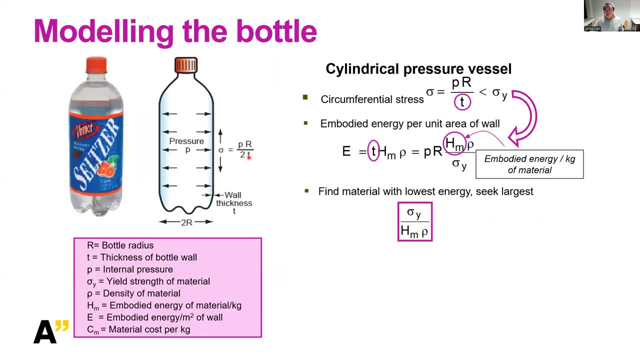 right, you need to also always minimize the material cost. that has been really environmental driving force for many businesses. uh, if you just add this into consideration, as you can see, and i think we don't need to derive for the cost situation- yeah, you can basically memorize the material index for cost related. 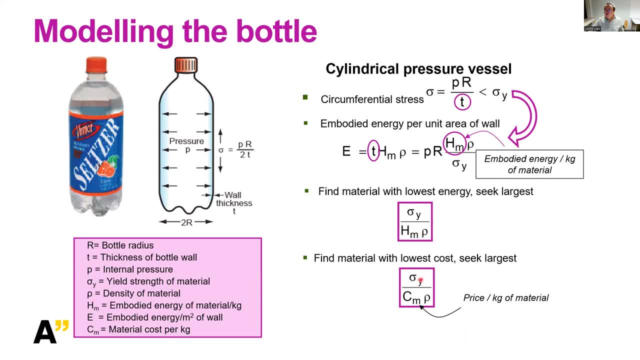 issues and here, as we are thinking, looking for the yield strength, basically we just replaced hm by cm, which is the material cost per kilogram, and that's your second, basically, material index. now we have two material index and you can easily think about how to solve this issue. so well, what we need to do. 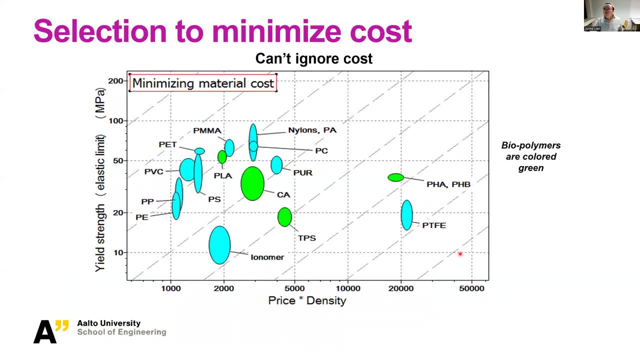 is basically to construct a um trade-off function, right, and then you, you, you will need to plot this and then you can further basically go with the plan penalty function and make a detailed selection. yeah, so here i'm showing you everything here with the, with this, uh, with this. now about the: 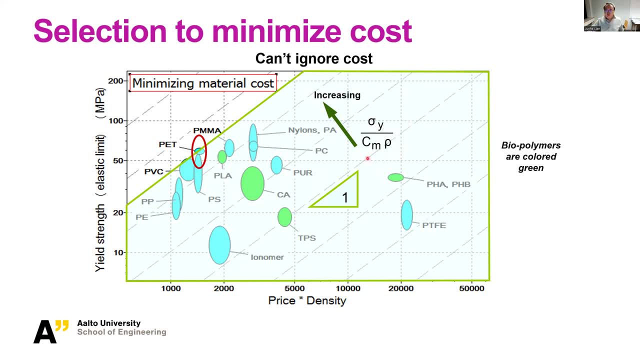 uh, cost situation only. yeah, so here we see, if we just take the x-axis as price times, density as the cost only, and the y-axis as yield strength, you you will now find the pt. so pt is right here. that's why we in the reality, at the moment at least most of these bottles, are made of pt. 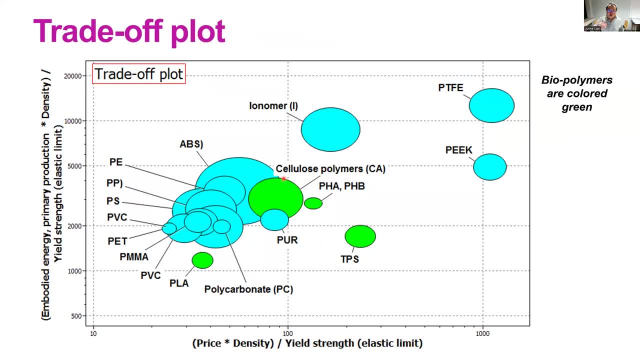 and now take consideration about costs and also the equal impact altogether, you can construct such a trade-off plot. So here is basically the price, the price over yield strength, and here is the embodied energy over yield strength. And you can see, this is our trade-off curve. 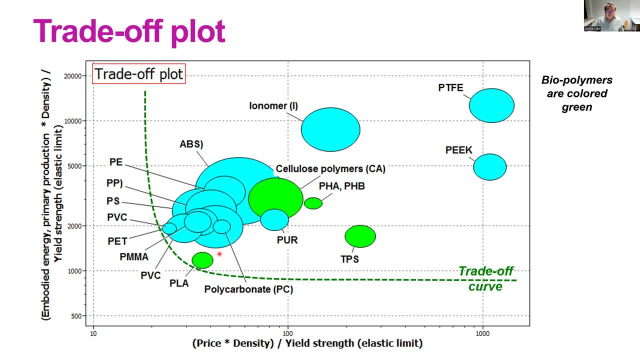 our trade-off in front. And so here is PET. So you can see here and here's PLA. Yeah, exactly, They're on the front. If we don't consider price, we will definitely take PLA, And if we take more serious about price, 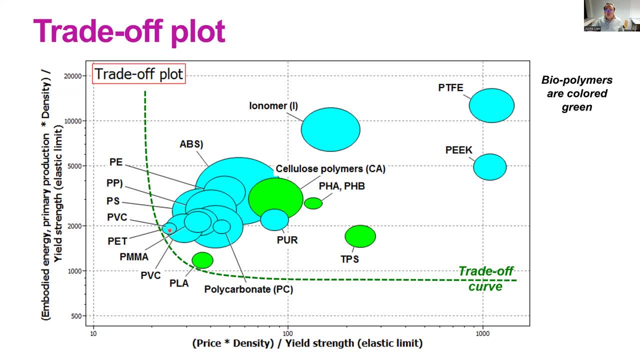 less about environmental impact. of course, PET is a pretty good choice. So, so far as you can imagine, we're more taking this, the pricing, into consideration, but now with all this government influence and also kind of good policies for using environmental friendly materials and so on, 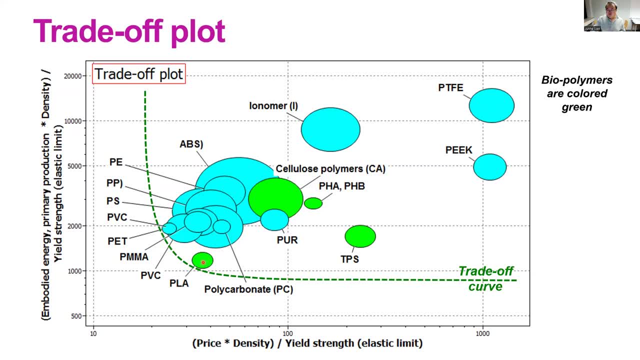 I could imagine we will more and more go towards such a direction. So if you formulate a penalty function, you can imagine the alpha value will be significantly influenced by that. That will make finally decide you will go a penalty, a penalty function like this: 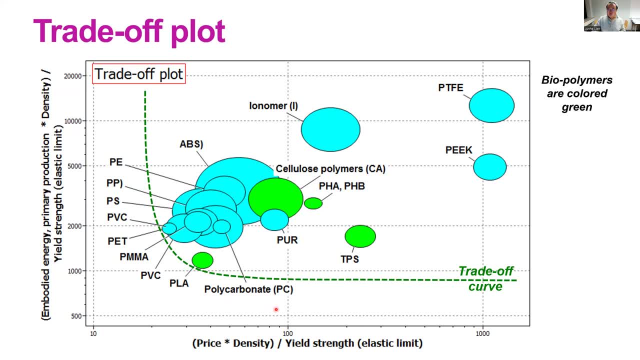 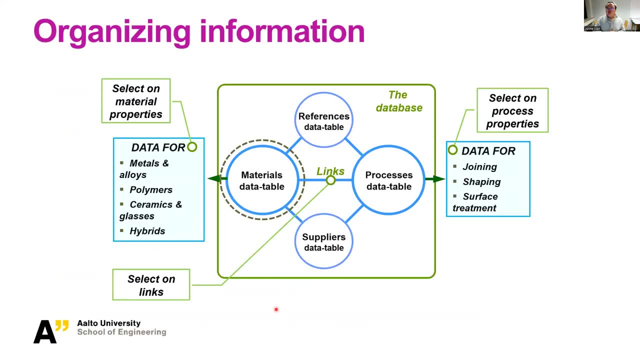 or you would go with like that, That will decide basically different materials. All right, I think that's the example I would like to talk to you, And you will learn much more from the book and also from your task. You also got a feeling about the use of audit. 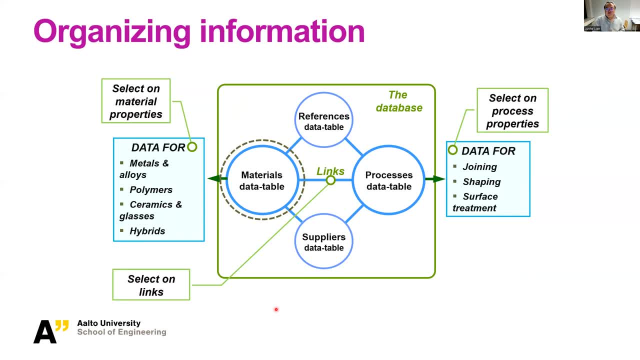 And the last thing I want to talk about is these processes, And here I'm showing you one diagram We have, I think, showed probably at the beginning of the course, maybe the first or second course. So this is the structure of the information. 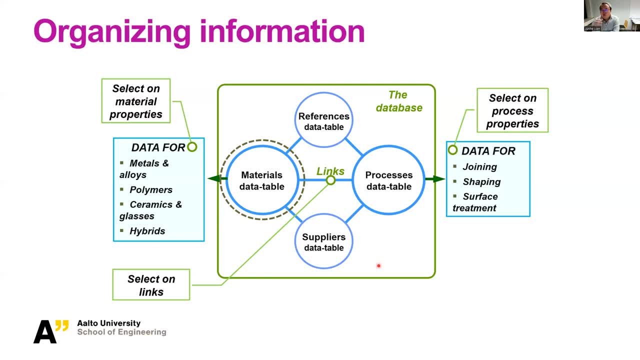 What we should do when you do the material selection and what the GDU pack is organized to, to to let us use. Yeah, we focus a lot about the material database and we were basically doing so many things in in the past few weeks, right, right here. 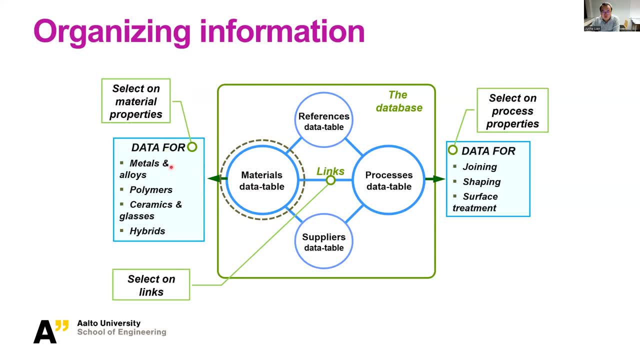 You will also learn all the different materials, from hybrid, from metal alloys to hybrid, And today we're going to talk a little bit about the processes. So, as you can see here- and the processes data table is organized very similar to the materials data table- 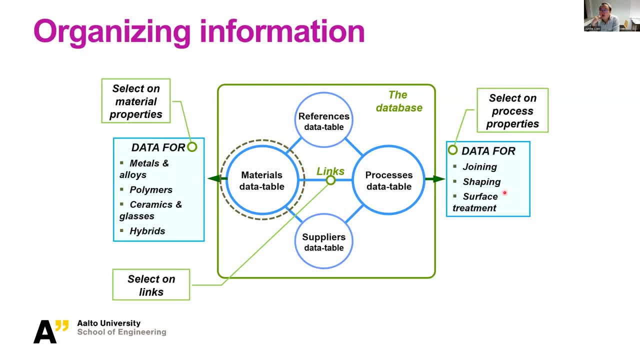 And you will see all these different kind of tree information in the next slide, And here, basically, I'm showing you three big families of processes. Yeah, So similar has materials. They are also three very important families, And so we have Johnny here first. 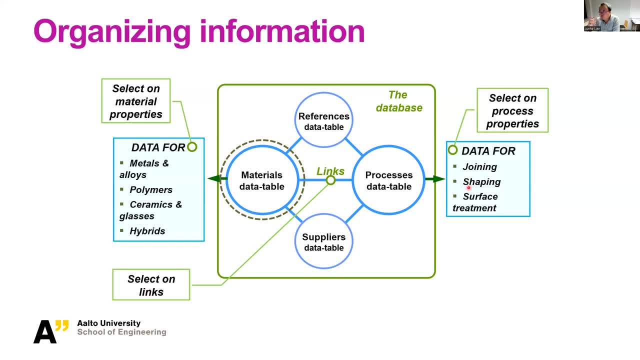 but maybe you can think about the shaping first, because you want to produce something like, for example, the core body. You will first try to get the shape of your, for example, the front panel, the bumper and also the door panel and all these parts. 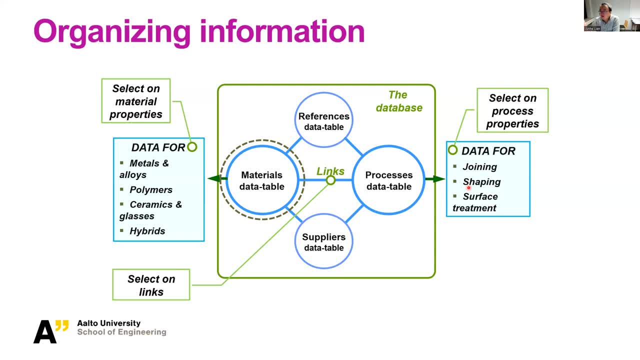 We need to first shape them. So there are many shaping methods, like casting- we have learned- and the material forming by stamping, by deep drawing, and all this and processes are used as shaping methods now And the joining is next. So after you get all this, 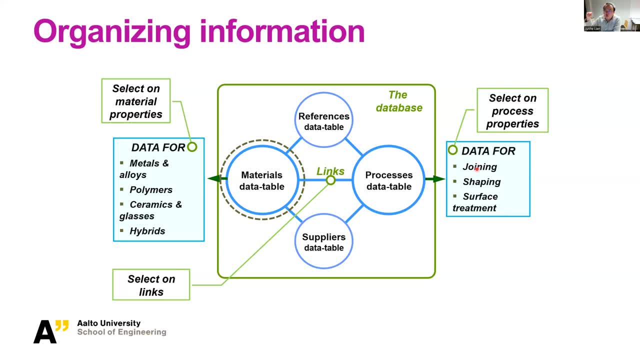 let's say door panel and the front panel and also bumpers. we need to put them into one piece, into the car, basically. And then you need all the joining technologies. Maybe you kind of recall we had a very detailed look at especially welding. 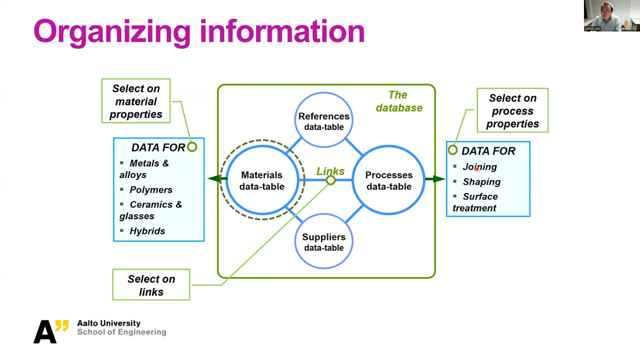 but also other joining methods. You are now resuming our course. And finally, it's about surface treatment. after you get the shape view and the piece joined together, when you consider how we're going to do the painting of your car, Should you do some polishing or make the surface more rough? 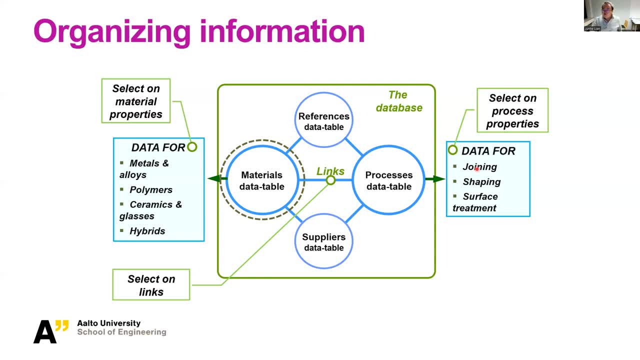 And those are all the surface related treatments. So after a certain treatment, basically your product is done. Now what we need to do is do do the selection of the image, the processes. So you're gonna use this way of shaping or the elevation, casting or deep join or stamping. 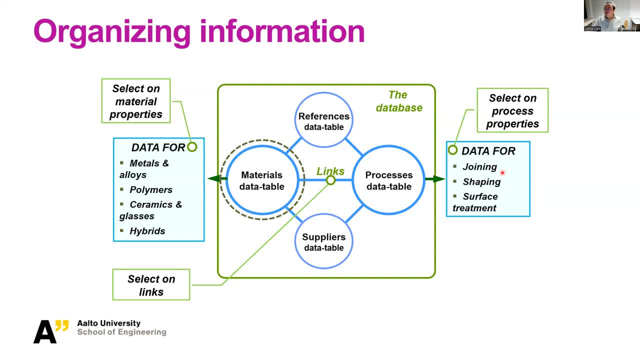 for joining you know. so this kind of laser welding or friction steel welding, and this will be the things you need to select. Of course, the most important thing is you need to select the links, So if the materials you select to fulfill the property requirements, 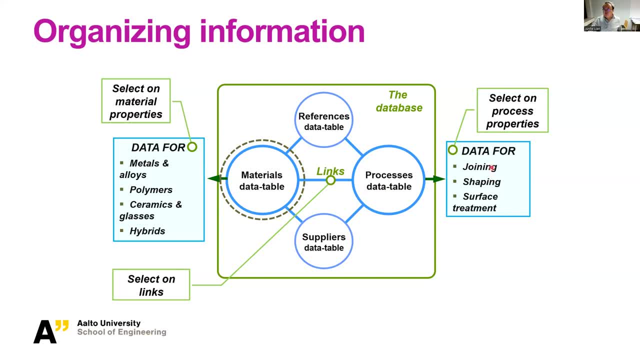 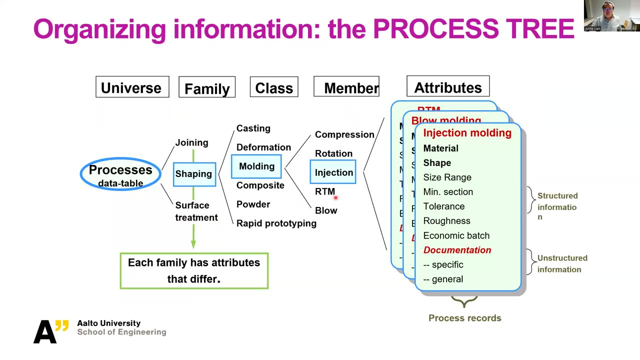 can be linked with the processes you would like to shape, join and search trim. So this is also a very important key selection you need to do So. you have to make sure they're compatible with each other, All right, so here I'm showing you this. 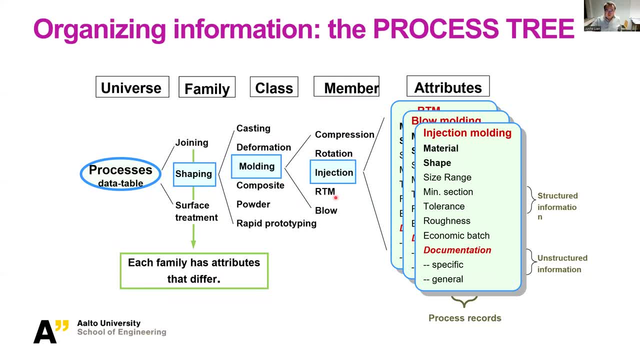 So organized information about processes, as we just discussed in the previous slide. They are also organized similar to the material tree. So this is so-called process tree. We have the family, these three big families, and then, when you go to classes for shaping, 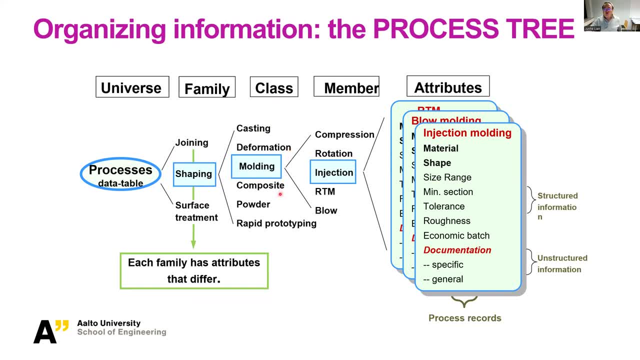 as you can see molding, casting, deformation and so on. And if you go more detail about molding you will see injection, blow and rotation and compression. And if you go to injection in more detail, you will see the specific process attributes.